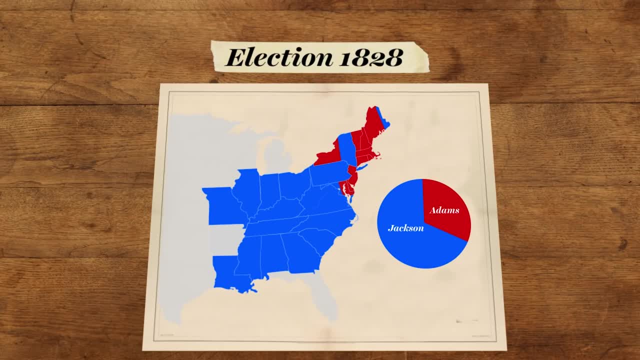 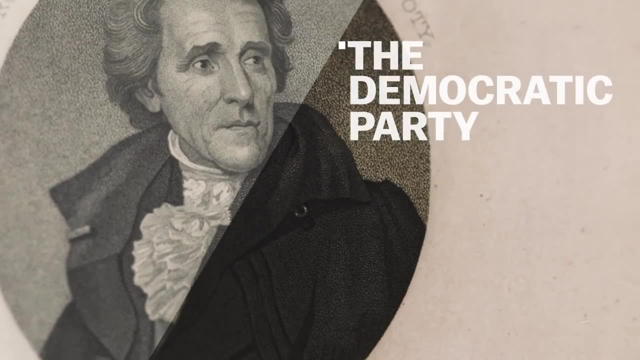 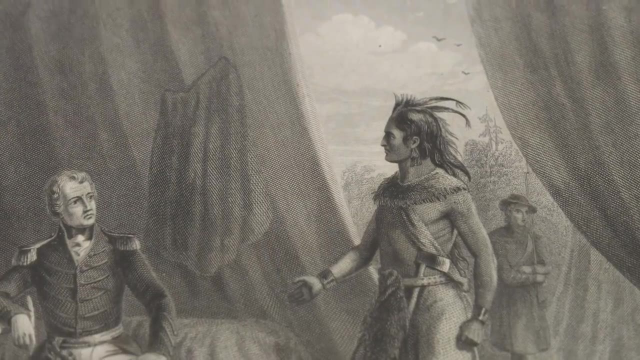 won in a landslide race. So his supporters argued that they, and not the old elites, represented the popular will of the country, and they started calling themselves the Democratic Party. Jackson's administration immediately began expelling Native Americans living east of the Mississippi River, an issue that defined the new administration. 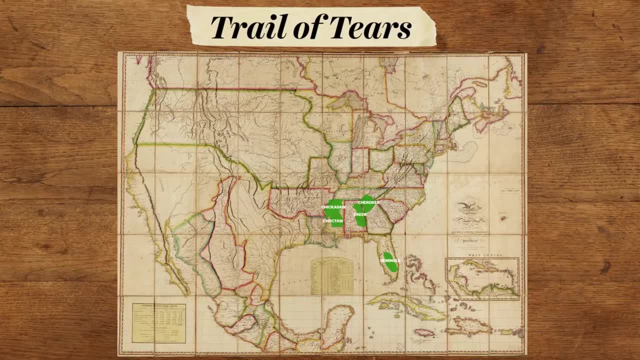 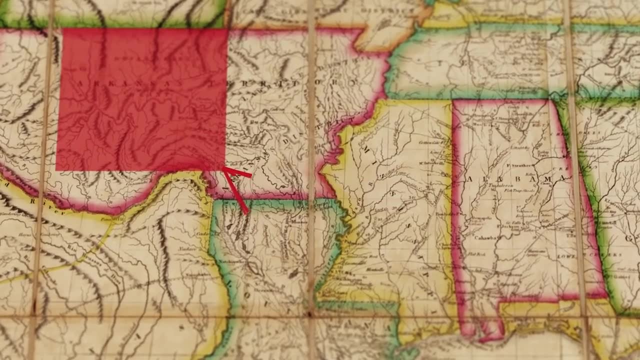 After he signed the Indian Removal Act into law in 1830, five large tribes were rounded up and forcibly marched into territories and camps further west. And the Democrats' ambitions didn't stop there. In the 1840s, the party adopted the 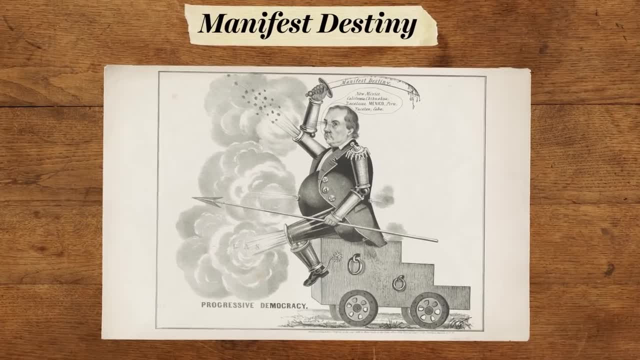 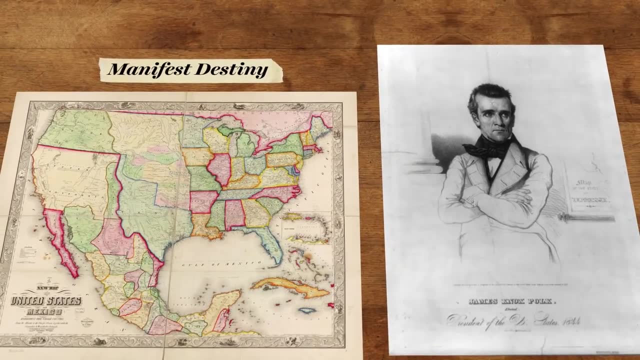 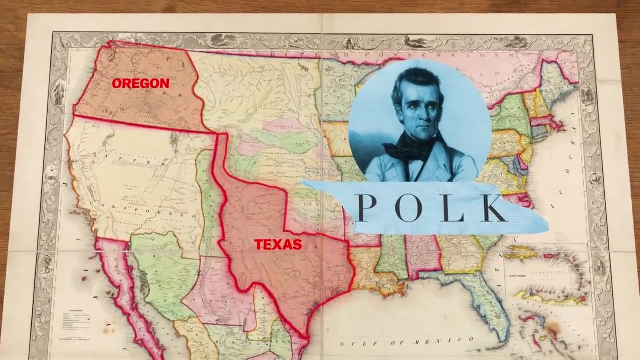 doctrine of Manifest Destiny—the idea that Americans- white Americans- were divinely entitled to dominate the whole North American continent. Democratic President James K Polk put this idea into action, massively expanding US holdings by annexing Texas, acquiring Oregon and winning much of what's now the Southwestern. 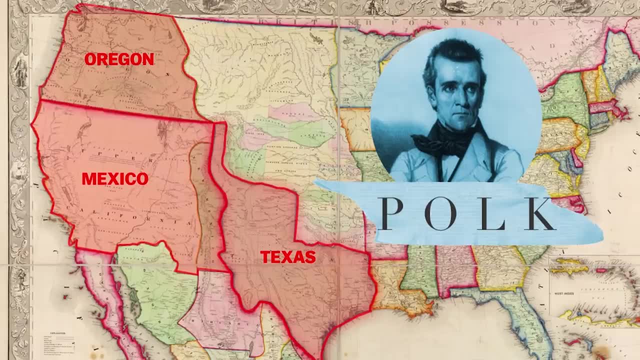 US in a war with Mexico. In the 1840s, the party adopted the doctrine of Manifest Destiny. It was the idea that Americans, white Americans, were divinely entitled to dominate the whole North American continent. National politics devolved into bitter controversy over whether new states entering the Union. 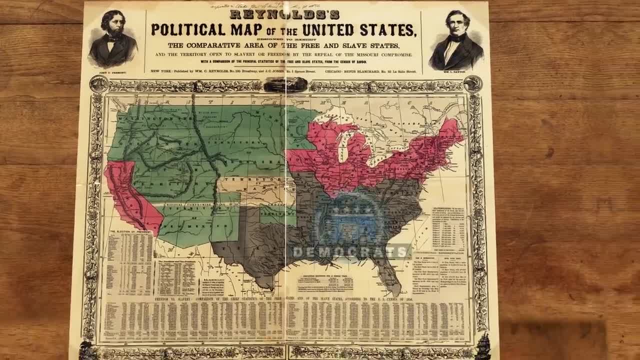 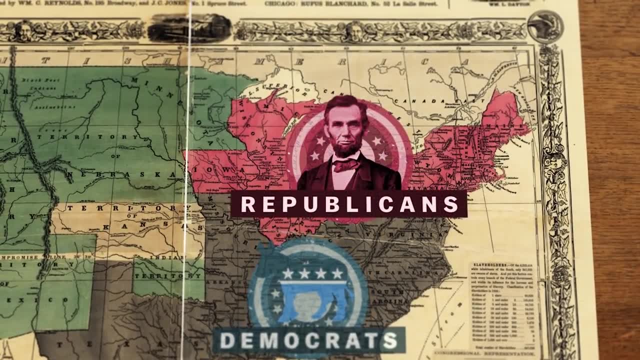 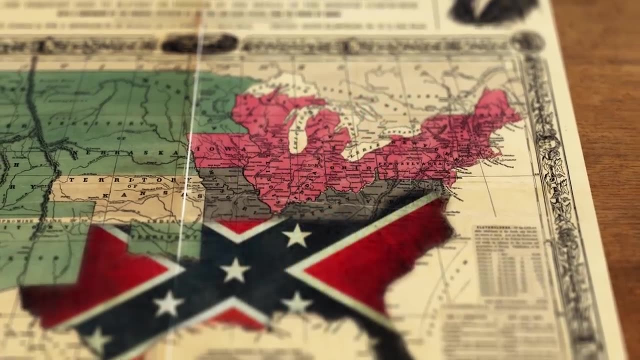 should be permitted to allow slavery. Democrats said they should, since their support base was strongest in slave-holding states. Yet a new northern party, the Republicans, sprang up in opposition to expanding slavery any further When Republican Abraham Lincoln won the presidency. the South seceded and the Civil War began. 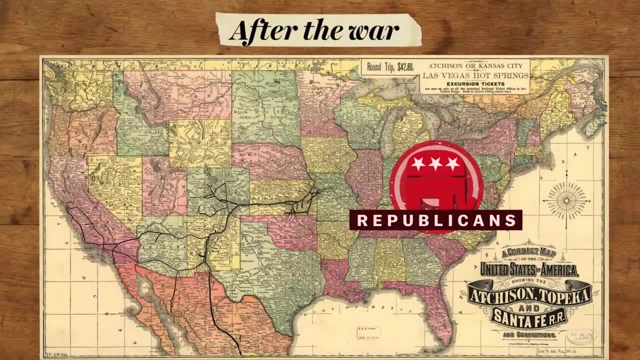 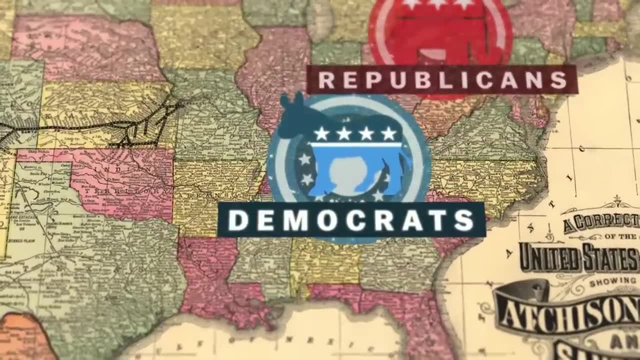 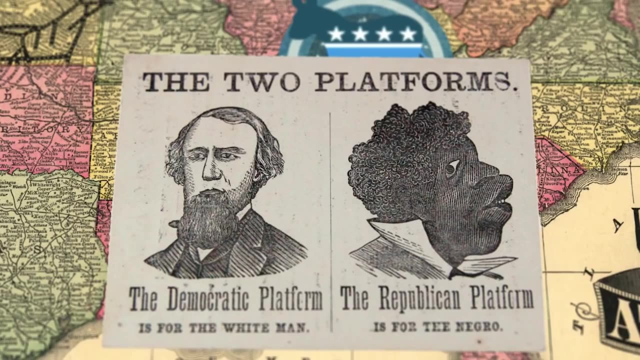 Once the Civil War was over, the Republican Party was bitterly unpopular among white southerners who wanted to maintain supremacy over former slaves. So the Democratic Party promised to limit federal government intervention on behalf of black citizens. Democrats became effectively the only political party in the South aided by intimidation. 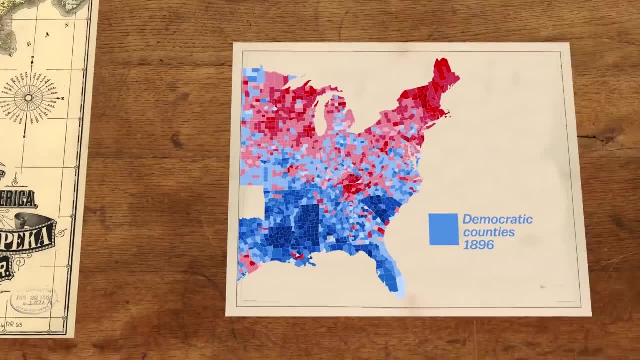 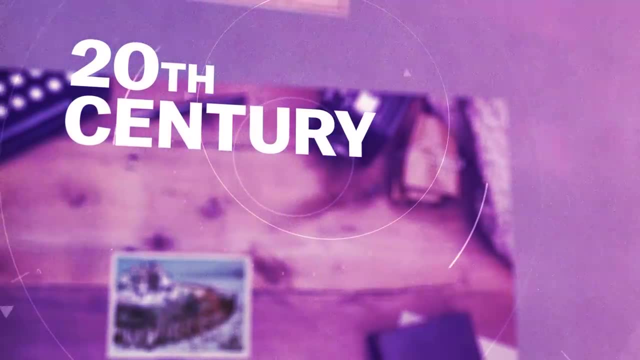 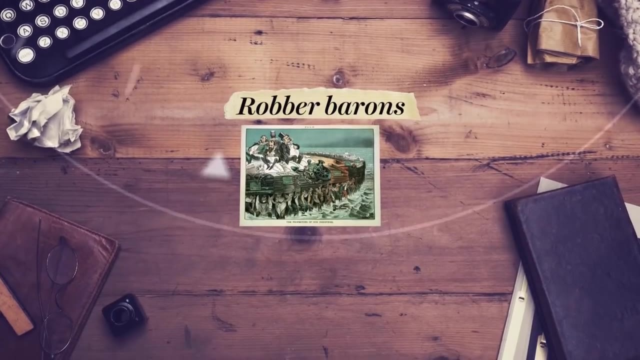 and suppression of black voters. Democrats also won on state and local levels, leading to the constant abuse of the rights of black citizens. As the 20th century began, the country was changing and the Democratic Party was changing too. A handful of individuals and corporations had grown enormously rich and powerful using 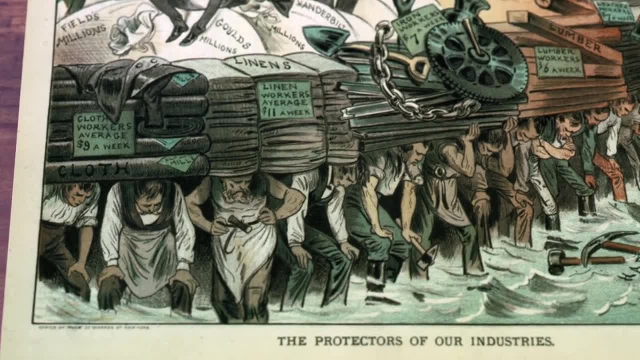 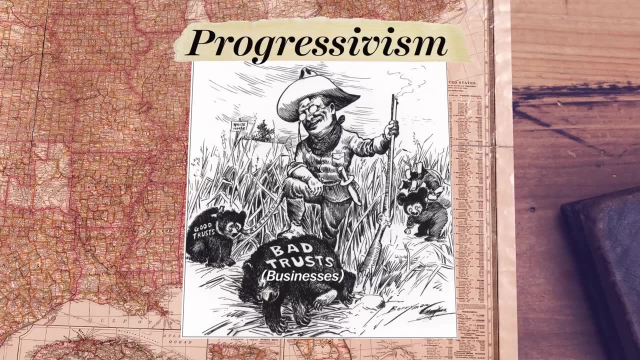 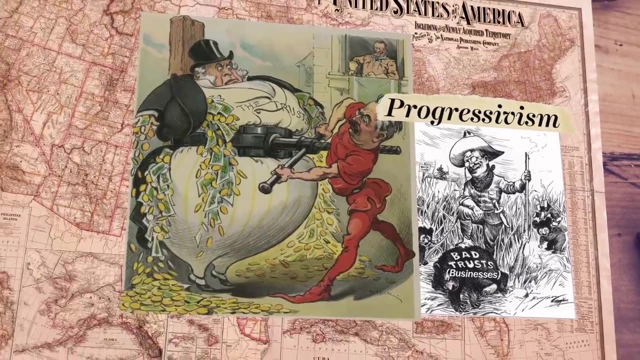 their vast fortunes to influence politics And as a reaction to this, some reformers began pushing an agenda of progressivism, arguing that the government should take more of a role in regulating big businesses and improving ordinary people's lives. At first, these progressive reformers were present in both parties, but it was Democrat. 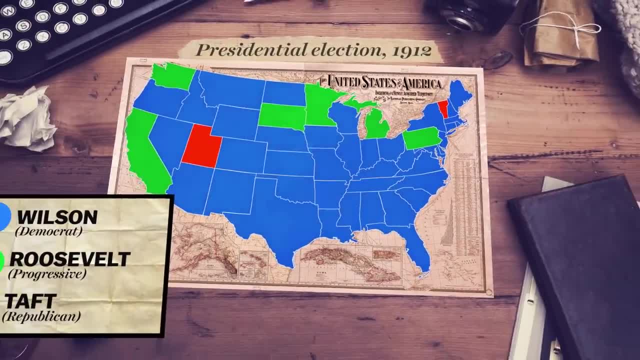 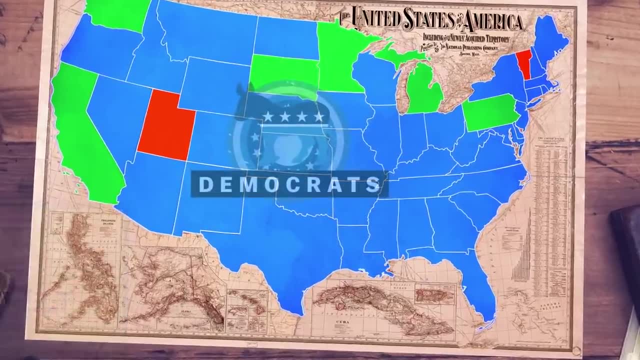 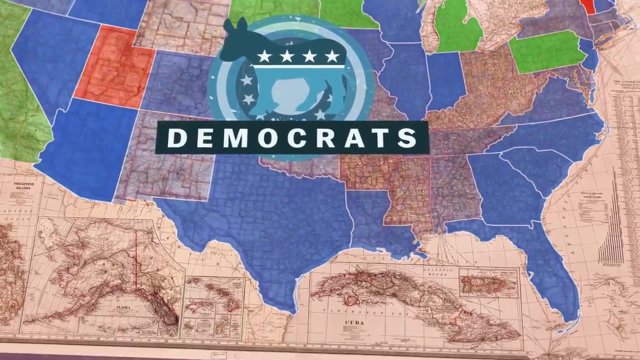 Woodrow Wilson, who won the presidency In 1912, the Democratic Party became the main home for progressives and the Republican Party became more the party of business. But it was the Great Depression of the 1930s that sealed the Democratic Party's new identity. 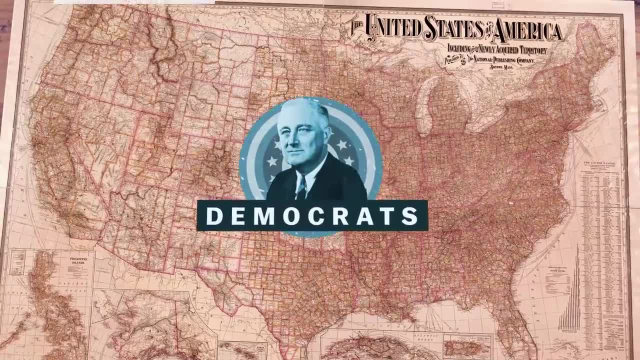 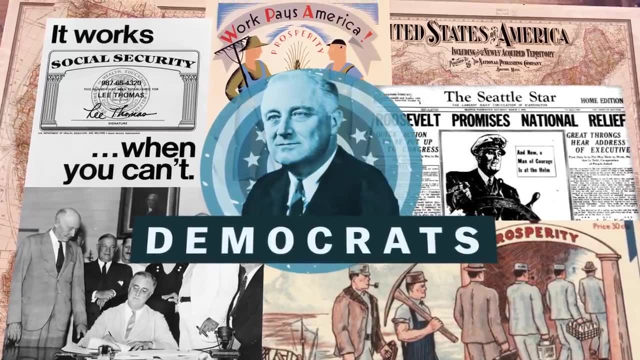 as the party of government activism. In an effort to combat the crippling economic situation, President Franklin Roosevelt signed what was then the largest package of domestic government projects in American history. In an effort to combat the crippling economic situation, President Franklin Roosevelt signed what was then the largest package of domestic government projects in American history. 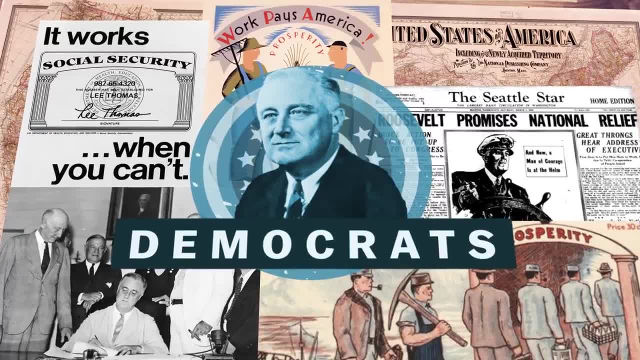 In an effort to combat the crippling economic situation, President Franklin Roosevelt signed what was then the largest package of domestic government projects in American history, calling it the New Deal, And in the process of doing this, his administration dramatically expanded the size of government. 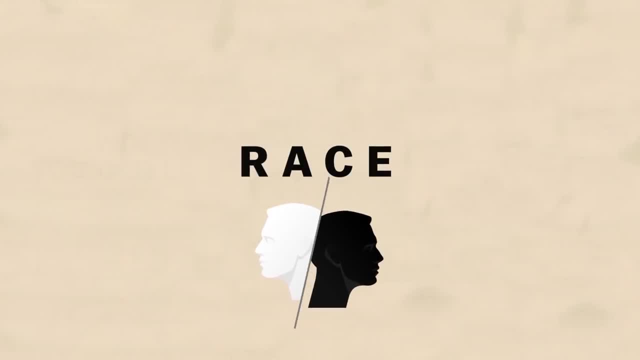 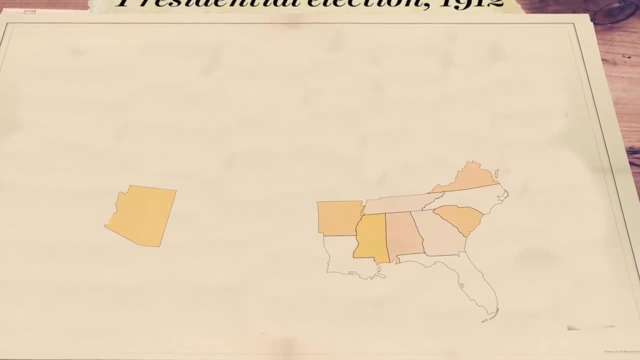 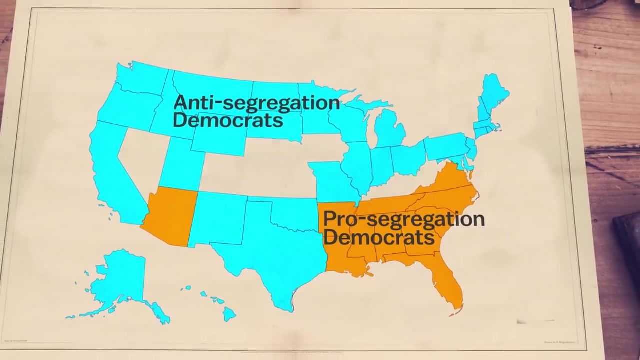 Yet the party was still split over race By the mid-20th century. it contained southerners who staunchly supported segregation, liberal reformers trying to end it and many politicians who were just happy to look the other way. But in 1964, when the Senate voted on the Anti-Segregation Civil Rights Act, this shows. 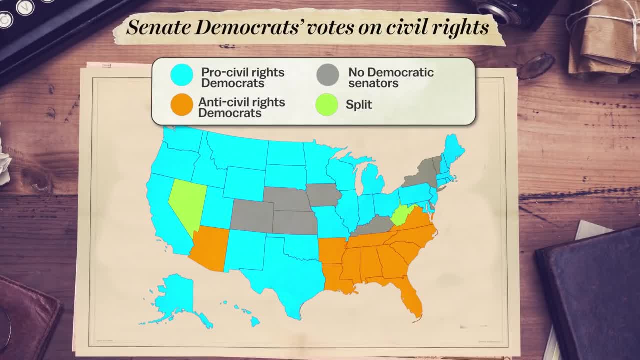 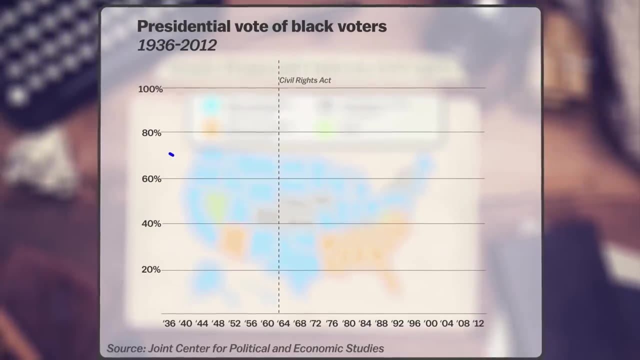 how the progressive reformers in the party had gained the upper hand, steering the party away from its racist past towards equality and social justice. But the Democrats in the South voted against the Civil Rights Act, remaining wedded to the idea of segregation. This chart shows the presidential vote for black voters. 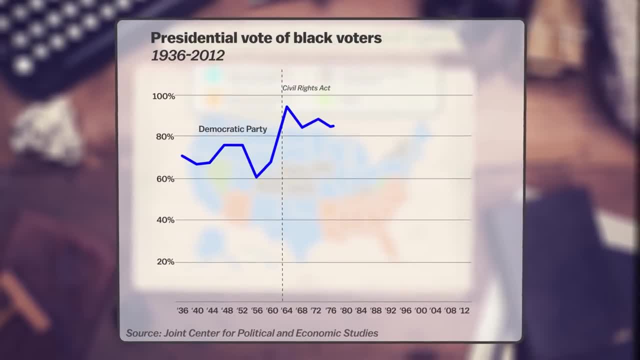 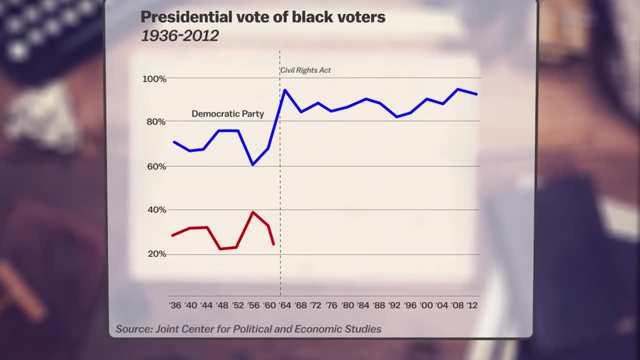 Around the 1960s, black voters who had already been moving towards the Democratic Party would begin overwhelmingly supporting the Democrats from then on And, conversely, the Republicans would take a huge hit among black voters. Meanwhile, white southerners moved away from the Democratic Party they had been loyal to. 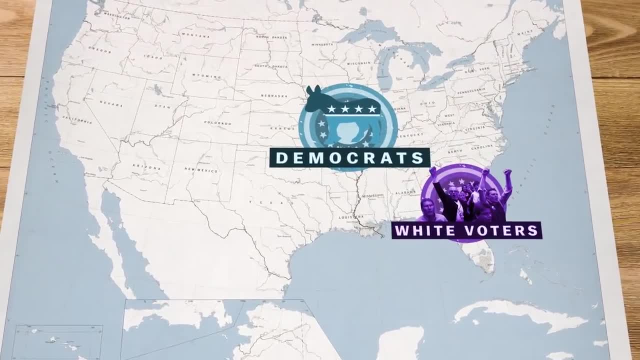 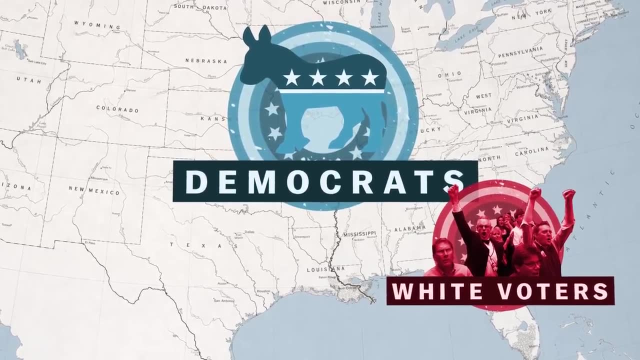 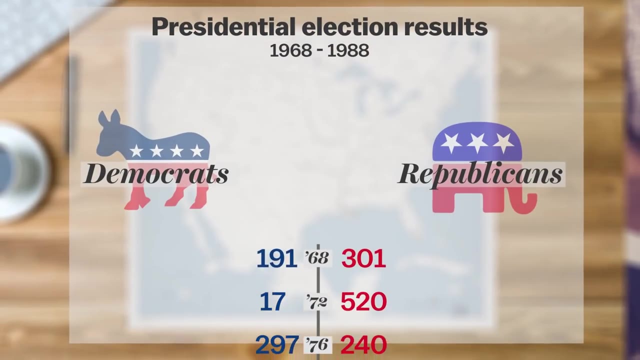 for so long, in part because of race, but also because of a suspicion of big government and a desire to defend traditional values against liberal activists. Democrats would go from dominating the South to losing almost all influence in the region. Thanks in part to this drop in popularity among white voters, Democrats started losing. 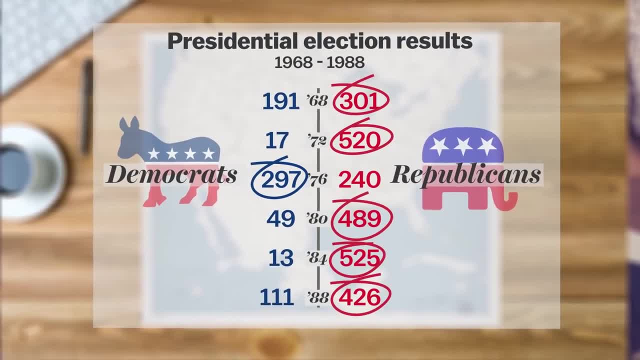 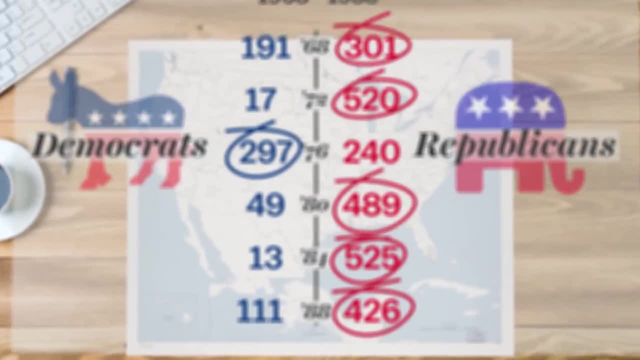 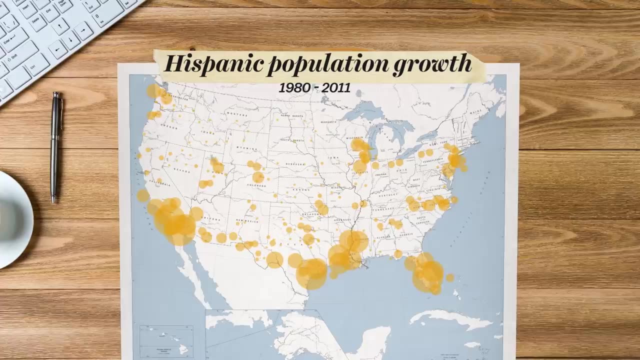 elections, often losing by huge margins. But demographically the US is becoming an increasingly non-white country and the Democrats have had a comeback, thanks in part to minority voters. The huge influx of Hispanic voters has especially benefited Democrats. These demographic shifts helped the Democratic Party once the advocates of white supremacy.